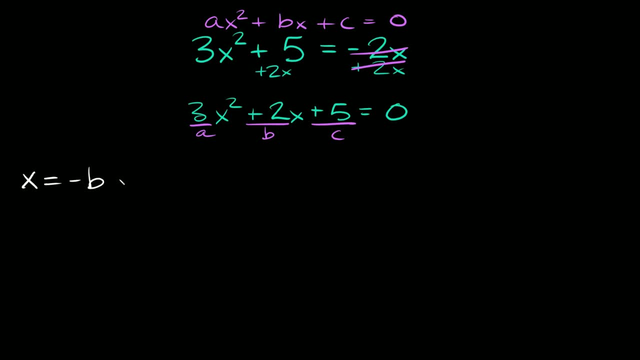 this beautiful thing right here. x is equal to negative b plus or minus the square root of b squared minus 4ac. I'm not done. All over 2a- All right now, I'm done. Okay. so this beautiful SOB is the quadratic formula, and now all we have to do is plug in our a, b and c numbers into the. 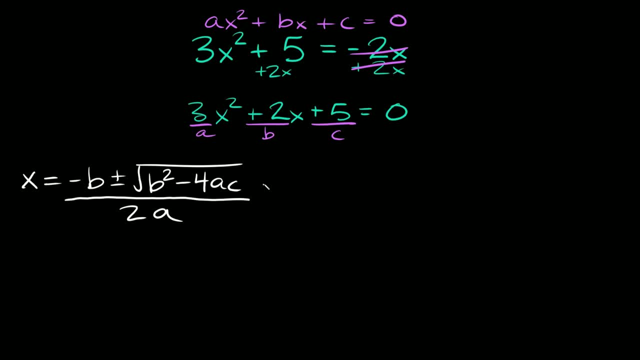 formula: Okay, so then here we're going to get that x is equal to- let's see negative, right? and then what's our b term? it's positive 2, so put a 2 right there, and then we're going to get plus or minus the square root of b squared, so that's going to be 2 squared minus 4ac, So a is 3 and b is equal to. 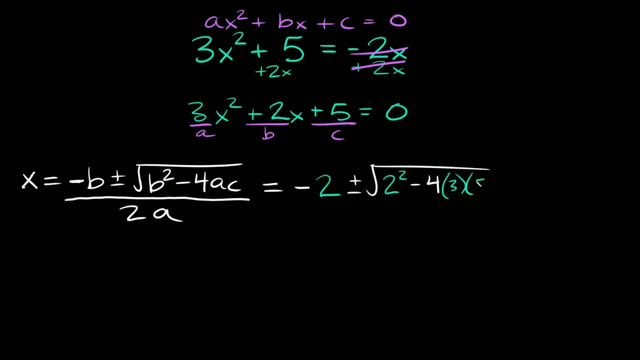 4 and c is 5.. Right, a is 3 and c is 5, and then that's all over 2 times a and a again is 3.. Okay, so now if we simplify this a little bit more, we're going to get that x is equal to. let's see: 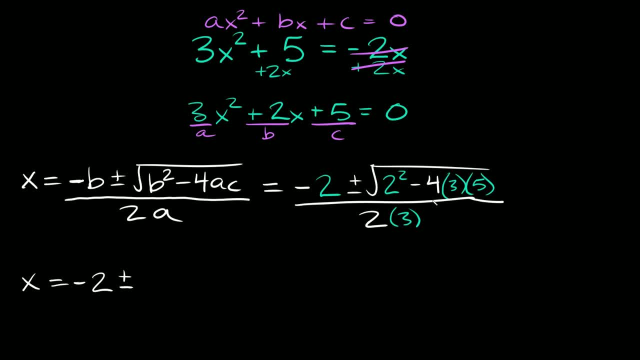 negative 2 plus or minus. right, negative 2 plus or minus. and then, inside the radical, we're going to get 2 squared, which is 4.. So the square root of 4 minus this, right here, 4 times 3 is 12, and 12 times 5 is 60.. Right, so minus 60.. Okay, and that's all over 2 times 3, which is 6.. 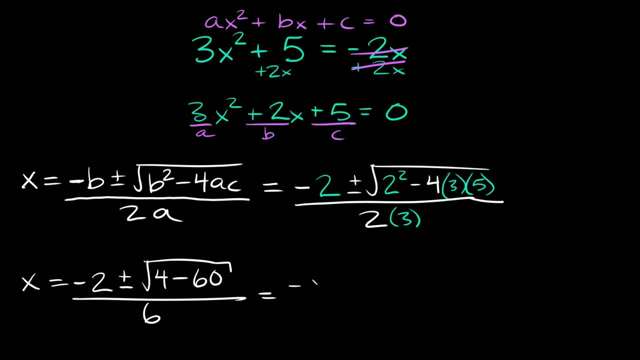 Okay. so then, if we simplify this again, we're going to get that this is equal to negative 2 plus or minus the square root of 4 minus 60, which is negative 56. right, negative 56, and that's all over 6.. Right, so here we have the square root of negative 56.. Now, whenever you have a negative 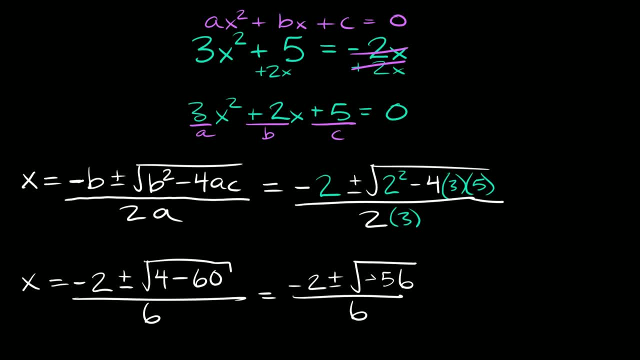 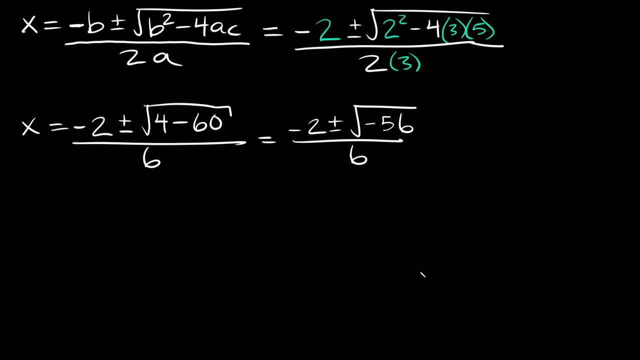 square root. That's obviously not possible, so that means we're going to have an imaginary solution here, right? So we just need to figure out what the square root of negative 56 is. So let's scroll down so we have a little extra root, Okay, and we can solve that off to the side over here. So 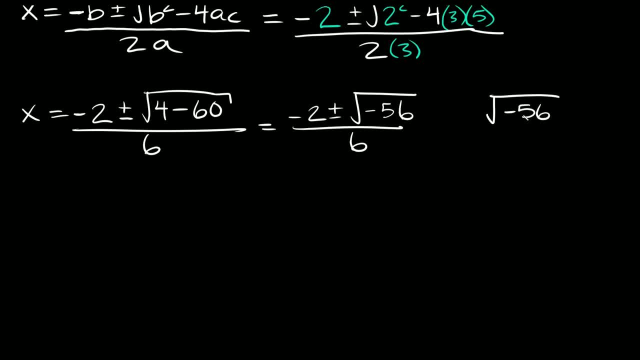 the square root of negative 56.. First of all, we can split up the number from the negative sign by writing it as the square root of 56 times negative 1.. Okay now, each of these get their own square root or their own radical. so we're going to write it as the square root of 56 times. 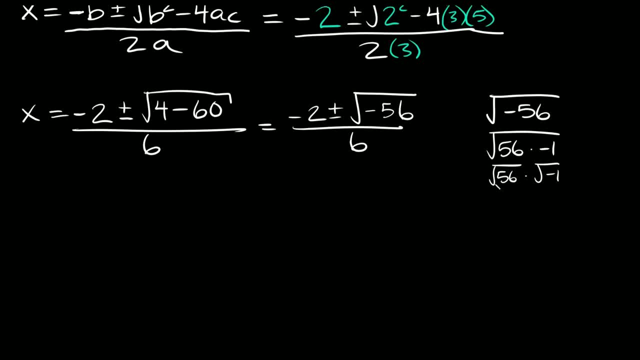 the square root of negative 1.. Okay, now the square root of 56. we can simplify this, right, and you want to use a perfect square if possible. So something like 4. okay, because 4 times 14 is equal to 56.. So we can break that down into the square root of 4 times the square root of 14. 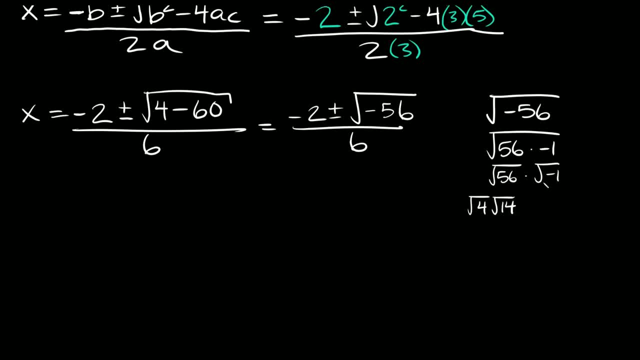 and then we're multiplying by the square root of negative 1, and the square root of negative 1 is equal to the square root of negative 1.. So the square root of negative 1 is specifically defined as i. Okay, so that's where the imaginary 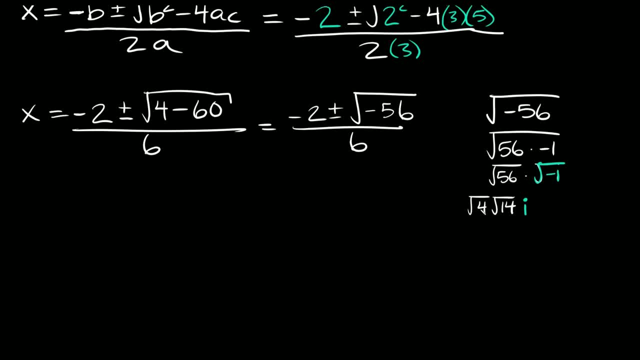 number symbol comes from right. So then, if we simplify this a little bit more, the square root of 4 is just equal to 2.. The square root of 14? we can break that down into 7 times 2, but that's not really going to help us, So you can just leave it as the square root of 14.. Okay, and then we still. 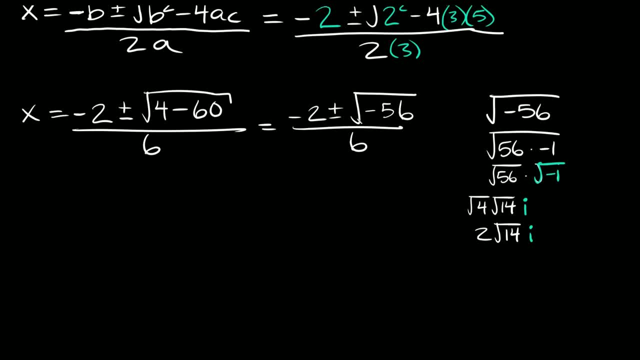 have our i right there. Okay, so the square root of negative 56 is equal to 2 root 14 i. So that's where the imaginary number symbol comes from. So then, if we simplify this a little bit more, So we're going to get negative 2 plus or minus the square root of negative 56, which is 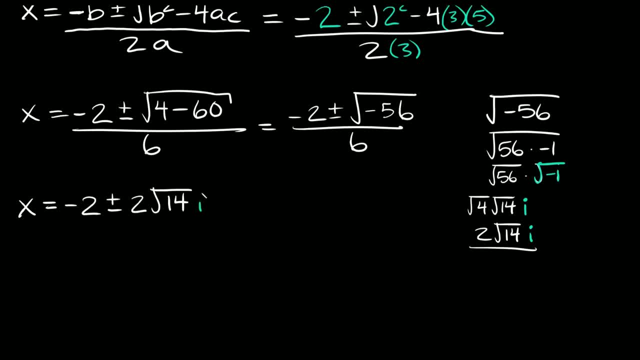 this right here: 2 root 14 times i all over 6.. Okay now, as you can see, we have a couple 2s right here, We have a 2 right there and a 2 right there and a 6 in the denominator. So 2 over 6 we can. 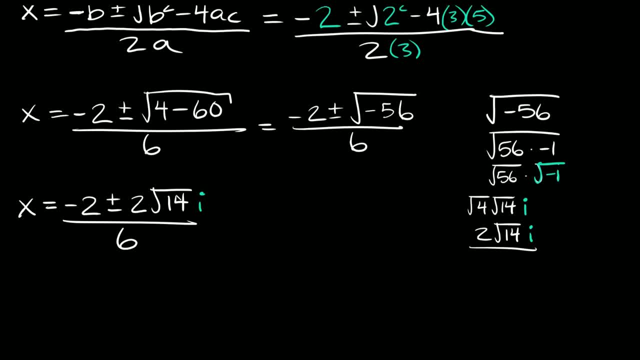 reduce that down to 1 over 3, right? So we can reduce that down to 1 over 3.. So we can reduce that down to 1 over 3, right? So we can rewrite this as 1 over 3.. So we're going to have negative. 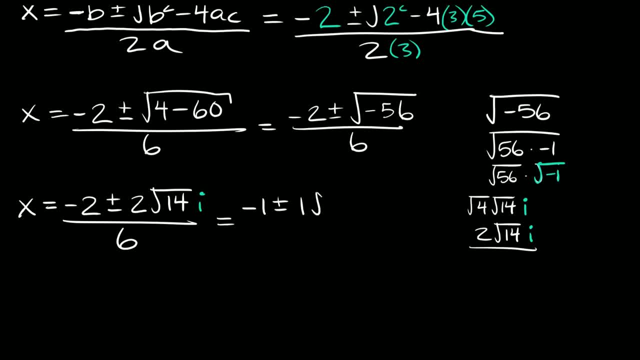 1 plus or minus 1 times the square root of 14 times i over 3.. Okay, but 1 times the square root of 14 times i is equal to just the square root of 14 times i, right, So we don't really need this.